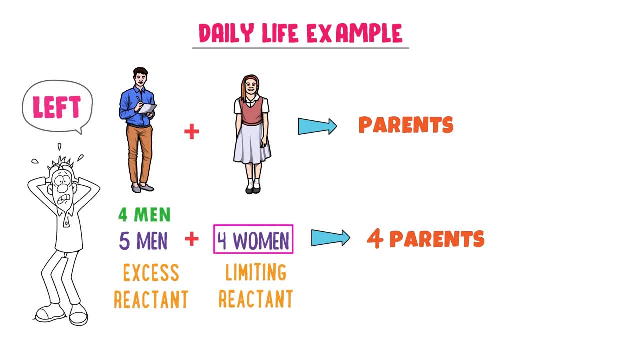 All these women are completely married to four men, so not a single woman is remaining, Hence it is a limiting reactant. On the other hand, out of these five men, only four men are married, and one person is still waiting for a woman to marry him, Hence it is an. 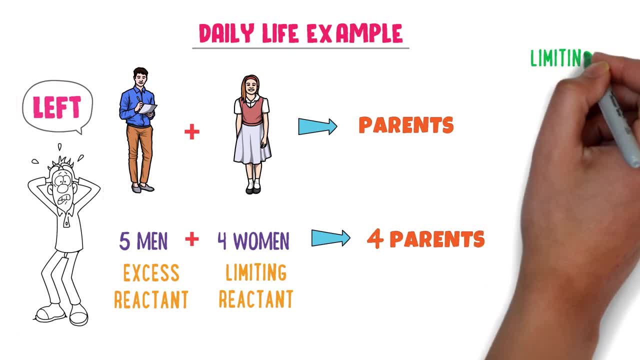 excess reactant. Thus remember that limiting reactant is the first reactant that is used up completely in a chemical reaction. Secondly, once limiting reactant is completely used, no more product can be formed. For example, when four women completely accepted four men, the process. 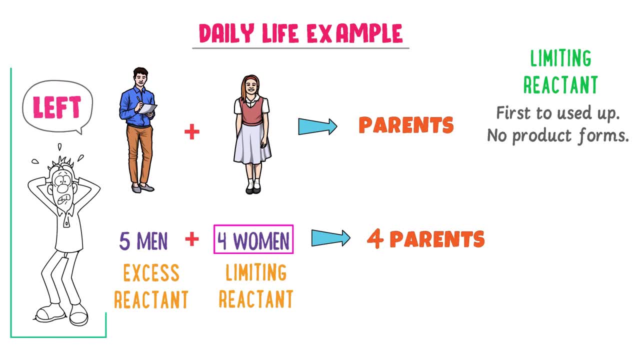 of marriage stopped, even though this unlikely person is still waiting, While the excess reactant is the left-over reactant. the excess reactant is the left-over reactant. Hence this kind of reaction is called limiting reactant, Or we can say that it is the unused reactant, For example, like this man is still waiting. 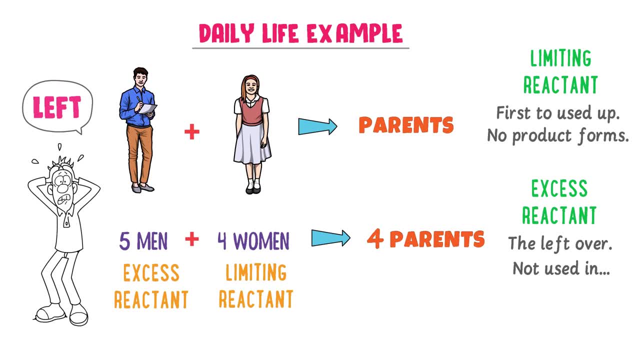 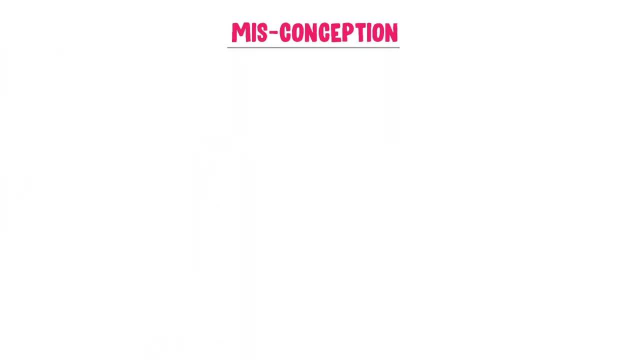 Thus remember the concept of limiting reactant and excess reactant. Now let me clear one biggest confusion or misconception about limiting reactant. A lot of people learn that limiting reactant is the least amount content in any chemical reaction. It is totally wrong and misconception. 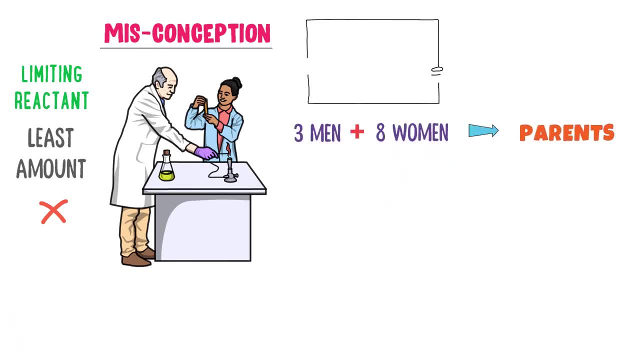 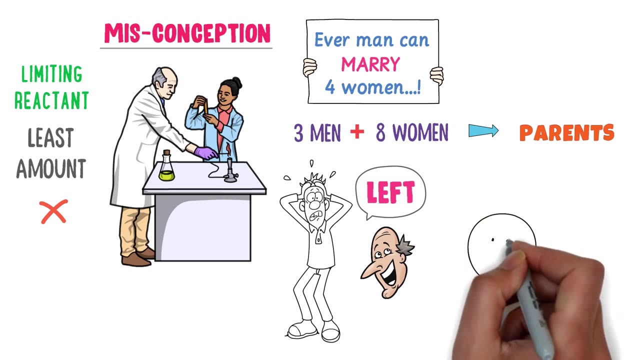 For example, consider three men and eight women. Now every man is permitted to marry four women, So the two men will marry eight women, and one person is still waiting. Believe me, I laughed a lot while writing this script and especially I feel sympathy for this unlucky man. 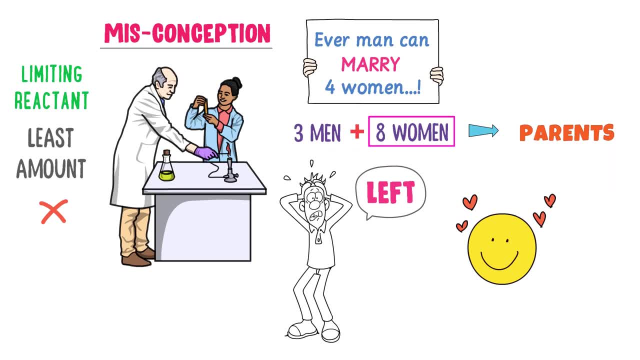 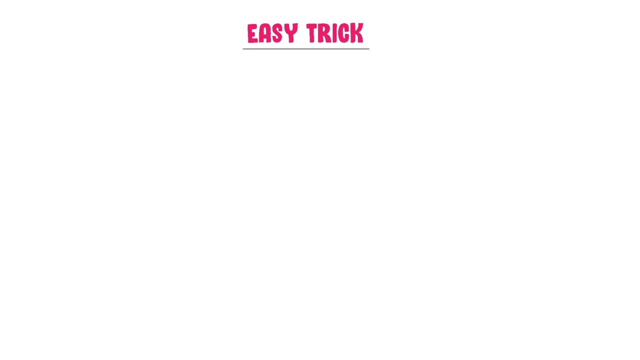 Thus, here, all the women are successfully married, Hence, being greater in amount, they are still limiting reactants, and men, being lesser in quantity, are still excess reactant. Therefore, remember this important concept about limiting reactant. Now let me teach you the easy trick of identifying limiting reactant and excess reactant. 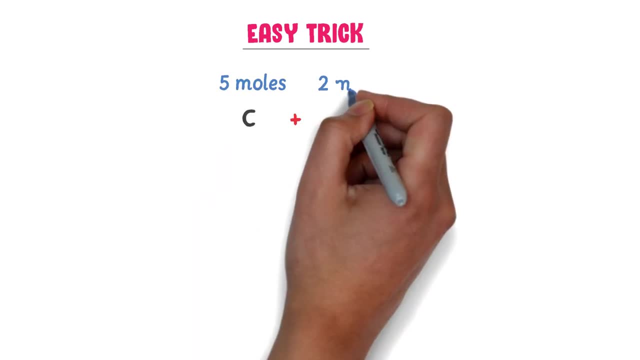 For example, consider five moles of carbon and two moles of oxygen. gas react together to form a reactant. Now let me show you how to form carbon dioxide gas. Firstly, I balance the chemical reaction. We can see that it is already balanced chemical equation. 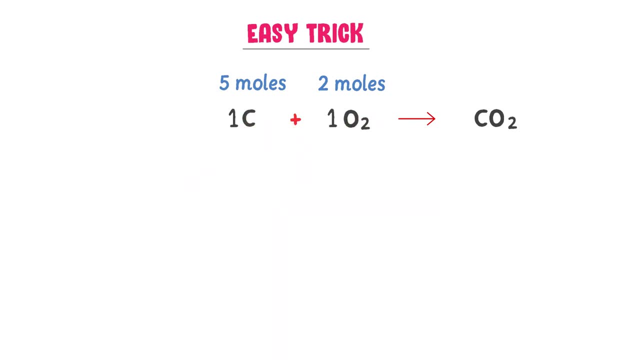 I write 1 and 1.. Now I will find the simplest molar ratio between carbon and oxygen. For instance, I divide the number of moles of carbon by its coefficient 1.. Similarly, I divide the number of moles of oxygen by its coefficient 1.. 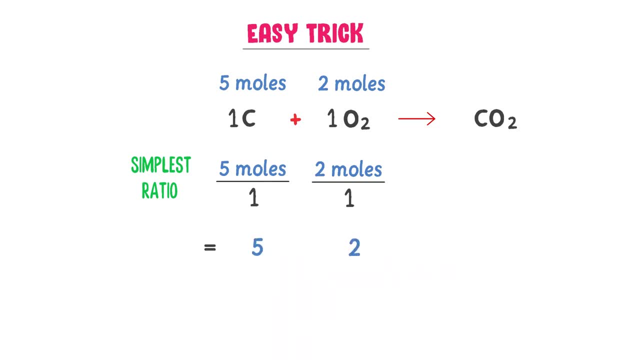 So I get 5 and 2. Here, 2 is smaller than 5. Hence we say that oxygen is limiting reactant and carbon is excess reactant. Thus, remember that the reactant which has the smaller ratio is the limiting reactant. 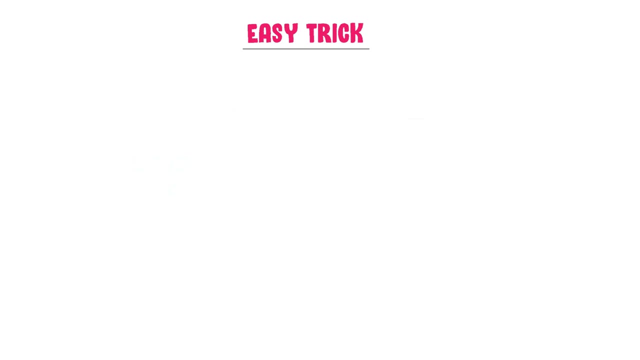 and the other one is excess reactant. Secondly, consider this chemical reaction. We are 3 moles of methane gas. react with 5 moles of oxygen. So we have 5 moles of oxygen gas. react with 5 moles of oxygen gas to form carbon dioxide. 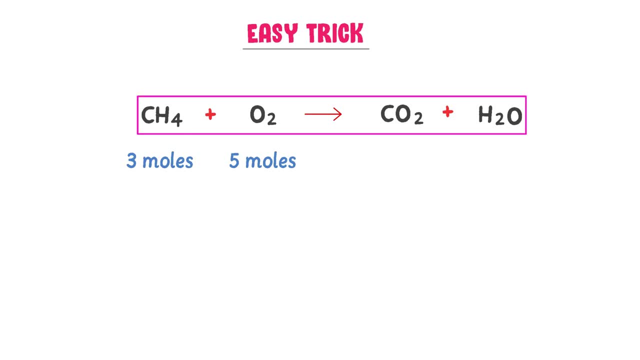 and water. I balance the chemical equation. I write here: 1, 2,, 1, 2.. Now I find the simplest ratio between methane and oxygen gas. I divide 3 moles of methane by its coefficient 1.. 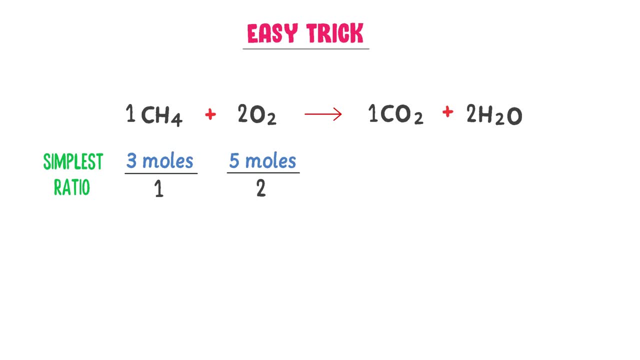 Also, I divide 5 moles of oxygen by its coefficient 2. So I get 3 and 2. Here 2.5 is smaller than 3. Hence oxygen gas is a limiting reactant and methane gas is an excess reactant. 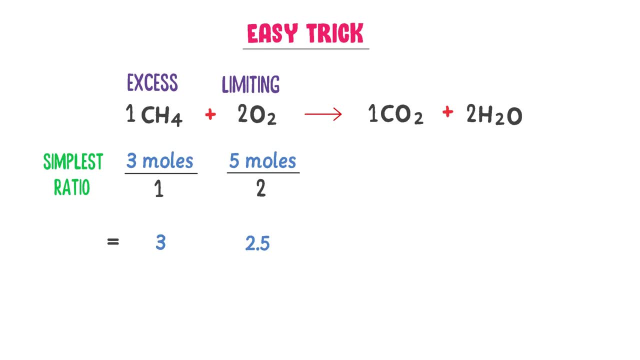 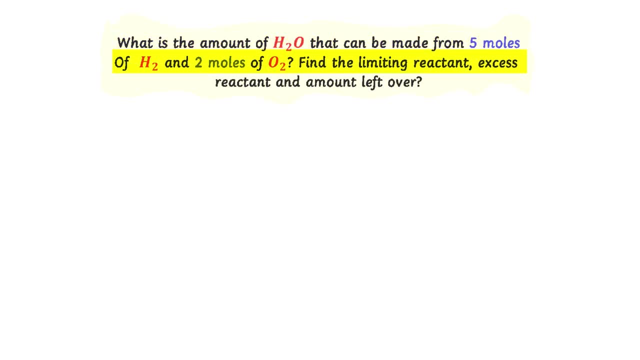 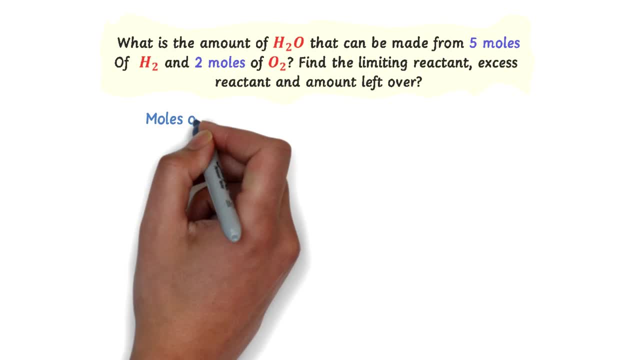 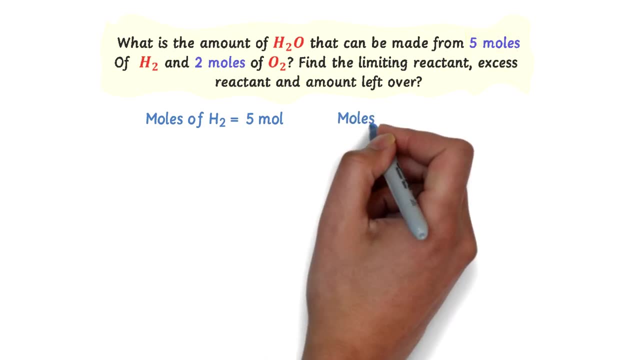 Well, firstly I write number of moles of hydrogen gas taken, which is equal to 5 moles. Also I write the number of moles of oxygen gas taken, which is equal to 2 moles. Then I write the balanced chemical reaction. 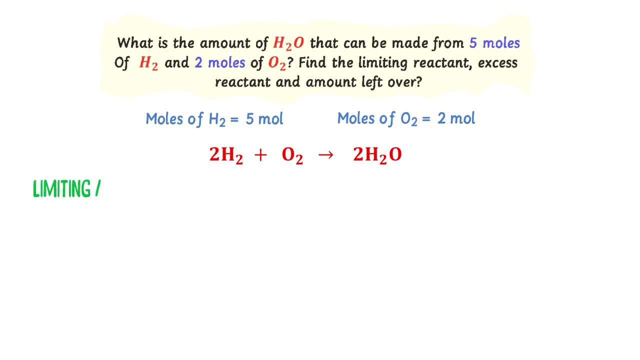 Now I am going to spot the limiting reactant and excess reactant in this chemical reaction. Here hydrogen gas and oxygen gas are reactants. I write 2H2 and oxygen gas. The number of moles of H2 taken is 5 moles and that of O2 is 2 moles. I divide the number of moles of 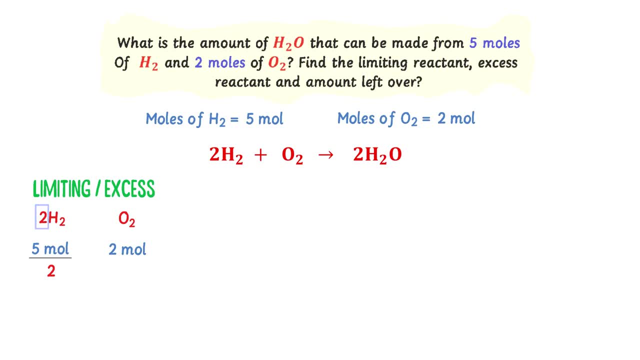 H2 by its coefficient and also that of oxygen by its coefficient. I do so in order to get the simplest ratio between them. I get 2.5 and 2.. Here 2 is a smaller number than 2.5. So oxygen is a limiting reactant and hydrogen is an excess reactant. Secondly, I calculate: 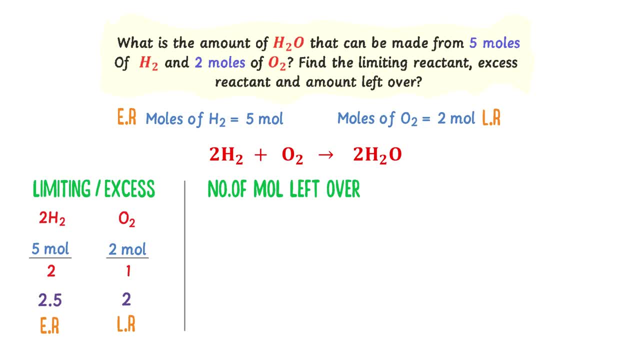 the number of moles or amount of excess reactant reactant left over in the chemical reaction. Well, I write the ratio of limiting reactant and excess reactant. The limiting reactant is oxygen gas, O2, and excess reactant is hydrogen. 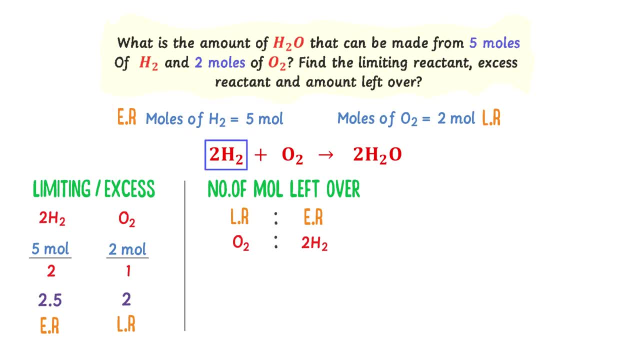 gas H2.. In the chemical reaction, the coefficient of hydrogen is 2 and that of oxygen is 1.. Let me repeat this important point: In the chemical reaction, the coefficient of hydrogen is 2 and that of oxygen is 1.. So the ratio of oxygen to hydrogen is 1 to 2.. Now listen. 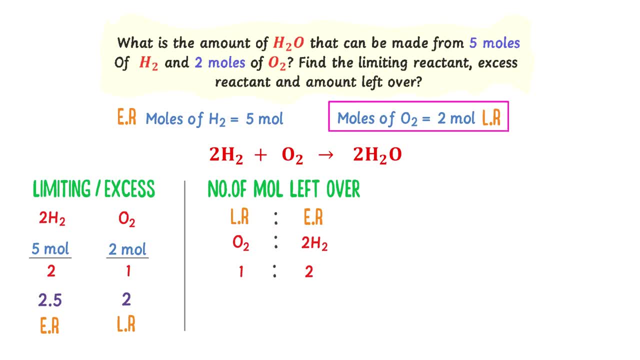 carefully. The limiting reactant is oxygen gas O2.. So its 2 moles is completely used in the chemical reaction. So I write here 2 moles of oxygen. Now, using this ratio, we can easily calculate the number of moles of H2 used in the chemical reaction. 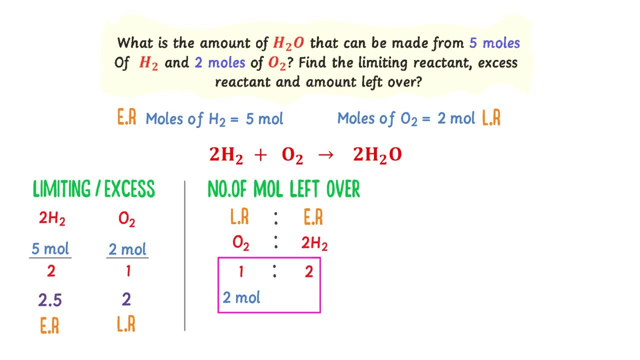 Now, using this ratio, we can easily calculate the number of moles of H2 used in the chemical reaction. So I write here 2, and for H2, I write x. After cross multiplication I get x is equal to 4 moles. Thus 2 moles of oxygen gas reacts with 4 moles of hydrogen gas. or we can say: 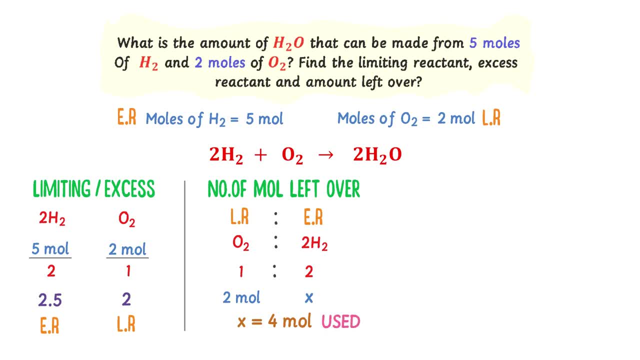 that 4 moles of hydrogen is used. On the other hand, we have taken 5 moles of hydrogen gas. So we subtract number of moles of hydrogen gas 2. I mean 5 moles minus 4 moles. I get 1 mole. So 1 mole of hydrogen gas is left over in. 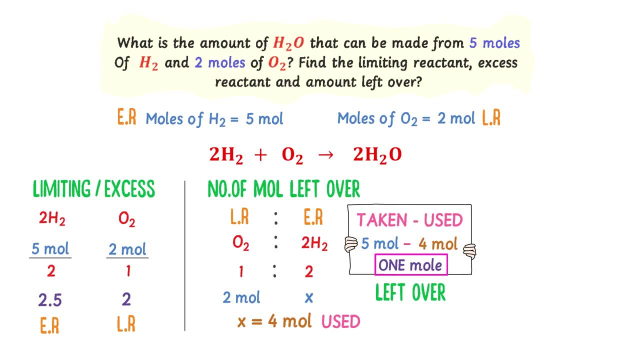 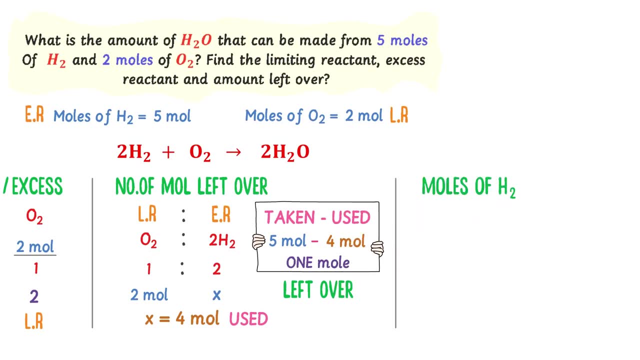 the chemical reaction. Thus the excess number of moles left over of hydrogen gas is 1 mole. The third step is to find the number of moles of H2O formed in a chemical reaction. I write the ratio between limiting reactant and product. The limiting reactant is oxygen gas, O2 and the 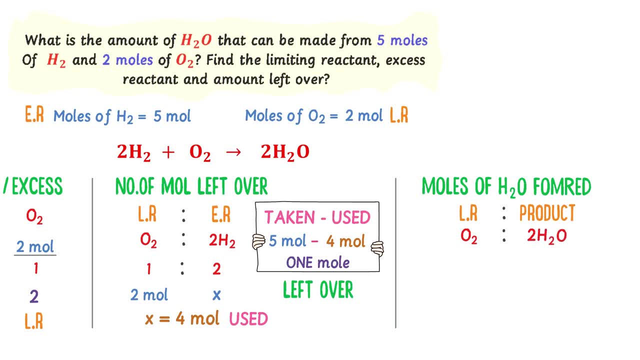 product is water, H2O. In the chemical reaction, the coefficient of oxygen gas is 1 and that of water is 2.. So the ratio of O2 to H2O is 1 to 2.. We know that oxygen gas, O2, is limiting reactant, and we have taken only 2 moles of oxygen gas. 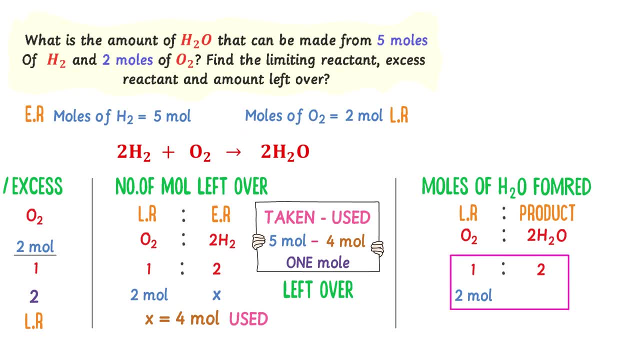 O2.. So using this ratio we can calculate the number of moles of H2O formed. Let it is x mole. After cross multiplication I get: x is equal to 4 moles. Thus the number of moles of water formed in this chemical reaction is 4 moles. Therefore we say that 5 moles. 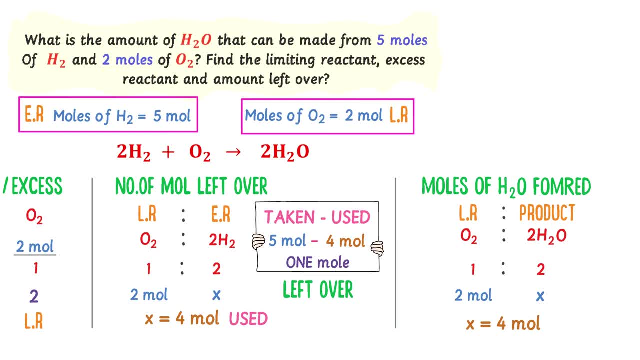 of hydrogen gas and 2 moles of oxygen gas react together to form 4 moles of hydrogen gas and 2 moles of water. Hence noted down this numerical question. Now let me teach you one last numerical: What mass of carbon dioxide gas formed in? 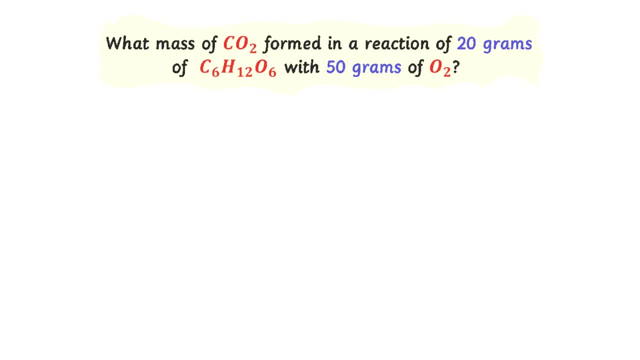 a reaction of 20 gm of glucose with 50 gm of oxygen. Well, in such type of numericals, firstly, we convert the given mass into number of moles. If you do not know how to calculate number of moles, watch our video, and its link is: 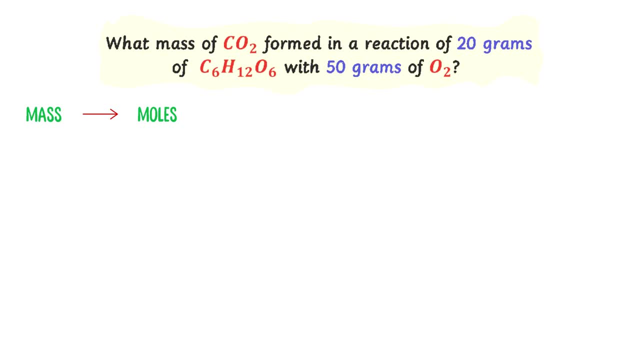 given in the description. Now I calculate the number of moles of glucose: 20 gm divided by the molar mass of glucose, which is 180 gm, I get 0.11 moles. Secondly, I calculate the number of moles of oxygen. 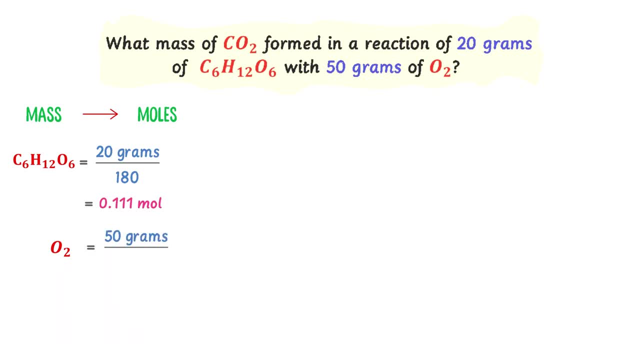 gas, which is equal to 50 gm, divided by the molar mass of oxygen gas, which is 32 gm, I get 1.5 moles. Thirdly, I write the balanced chemical reaction. The number of moles of glucose is 0.11 moles and that of oxygen is 1.56 moles. 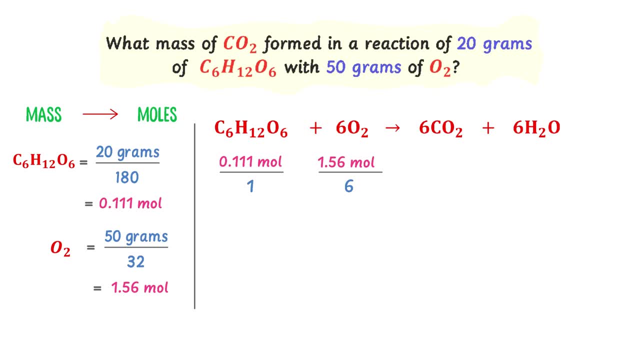 I find the simplest ratio between them. I get 0.11 and 0.26,. here 0.11 is a smaller number than 0.26, hence glucose is a limiting reactant and oxygen gas is an excess reactant. 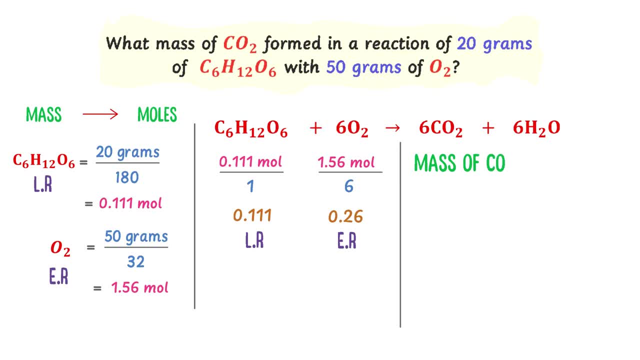 Secondly, I calculate the mass of carbon dioxide gas formed in the chemical reaction. I write the ratio between limiting reactant and product. The limiting reactant is glucose and the product is carbon dioxide gas. According to their coefficients, the ratio between them is 1 to 6.. 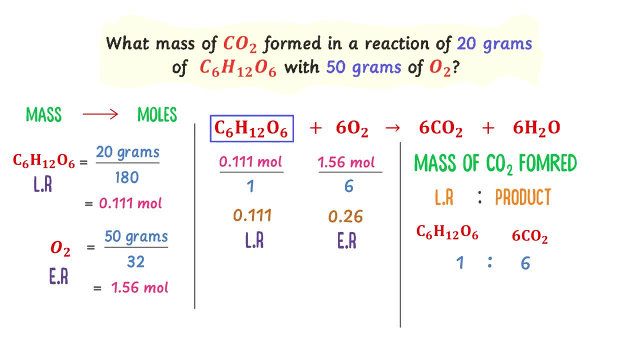 We know that the limiting reactant is glucose, and we have taken 0.11 moles of glucose, which is completely used in this chemical reaction. So, using this ratio, we can easily calculate the number of moles of carbon dioxide gas formed. 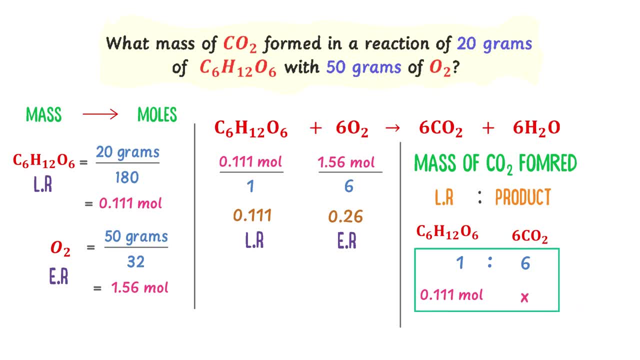 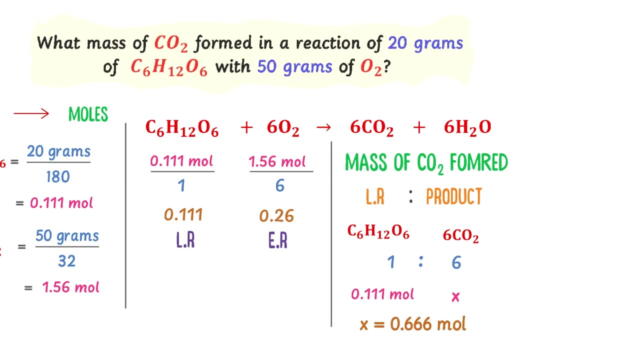 Thank you, Let. it is x mole. After cross multiplication I get x is equal to 0.66 moles. So the number of moles of carbon dioxide gas formed is 0.66 moles. But wait a minute. we are asked about the mass of carbon dioxide gas formed. 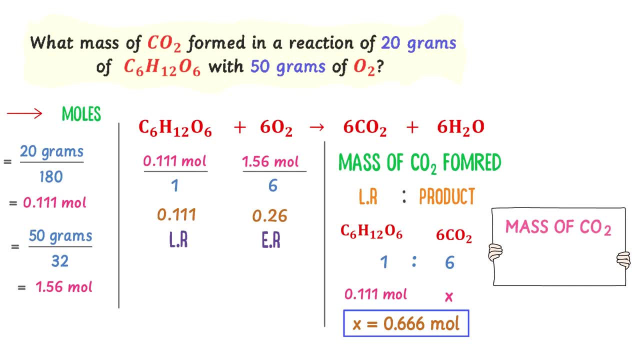 Well, we multiply the number of moles of carbon dioxide by its molar mass, which is 44 g, I mean 0.66 moles into 44 g. I get 29.3 g. So 29.3 g of carbon dioxide gas is formed in this chemical reaction.